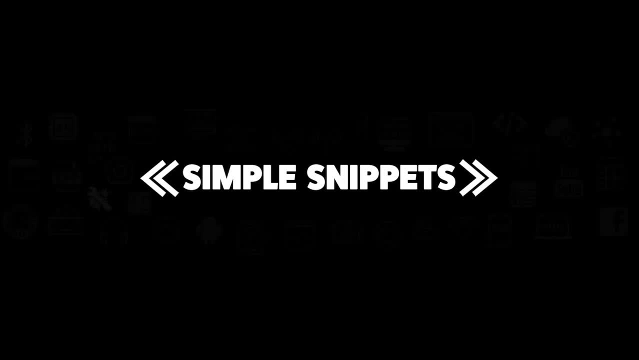 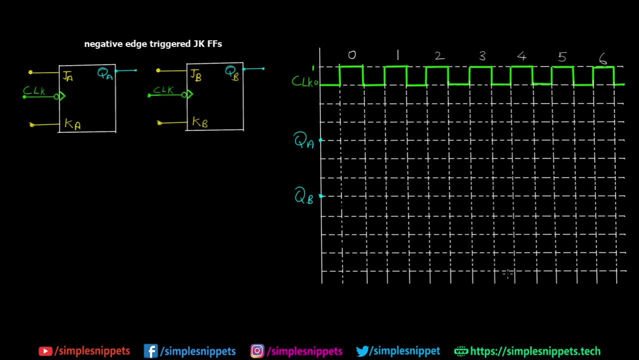 Yo, what's going on guys? Tanmay here for Simple Snippets and welcome back to a new video tutorial under digital electronics, and today's topic is gonna be the part 2 of introduction to counters. So in the part 1, we just took a very small and short theoretical representation. 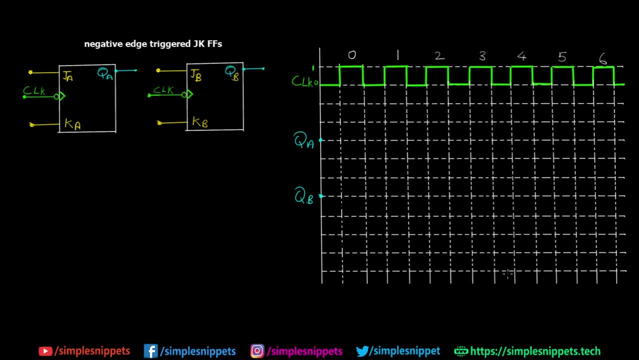 and explanation of what are counters, the application of counters and the types of counters. and I told you that in the next video, that is, in this part 2, I'll show you the circuit diagram. we'll also see the clock cycles and how the counter actually counts these clock. 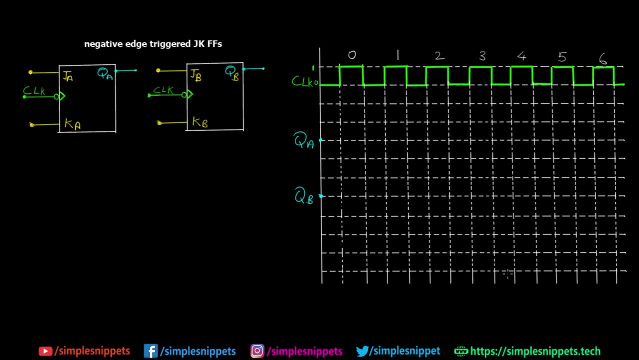 cycles. So everything is gonna be very clear in this video tutorial, so make sure you watch this video till the end and, with that being said, let's start off with today's topic. So, as you can see on the screen, I have two flip flops. You can see these are negative. 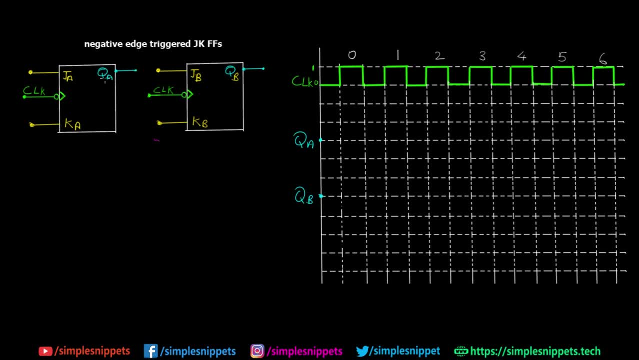 edge triggered JK flip flops. So we have J input, K input and we're just tracking Q as the output. And this is the second one: J, B, K, B. So this is the first flip flop, this is the second one and, since it is negative, edge triggered. 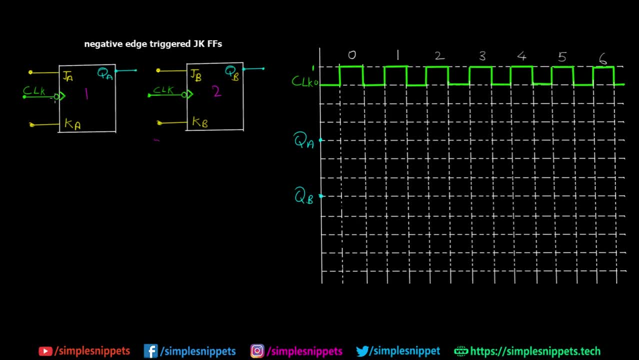 we have this bubble at the clock. So this bubble or this circle represents that it is negative and this triangle over here represents that it is edge triggered. Now we've already seen what is the different types of triggering methods and by negative edge triggered it. 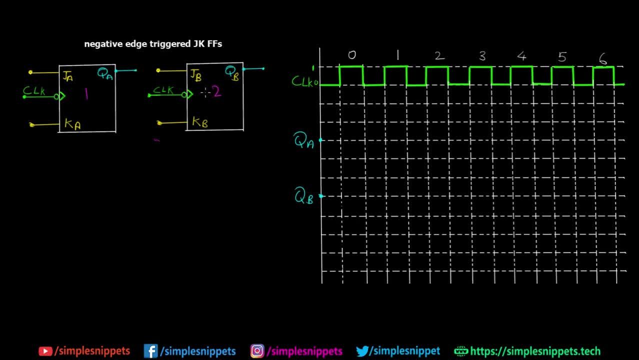 means that this JK flip flop and this JK flip flop will be activated on the negative edge or the dropping edge of the clock. So we know, if you see the clock over here, the negative edge is this one, right. So this is where the clock goes from one to zero. 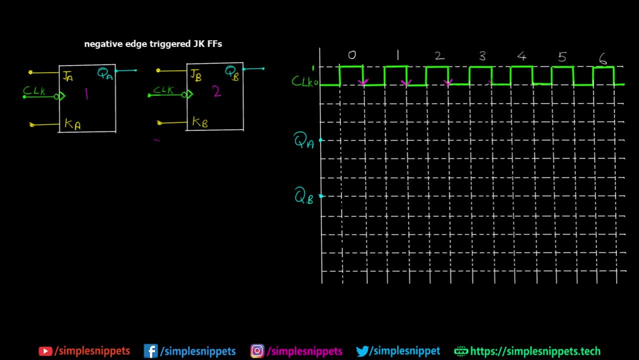 So every time there is a negative edge, our two flip flops are going to get activated, and that's when the switching is going to happen. And the reason why the switching is going to happen is because we are going to be passing the input as one and one for both. 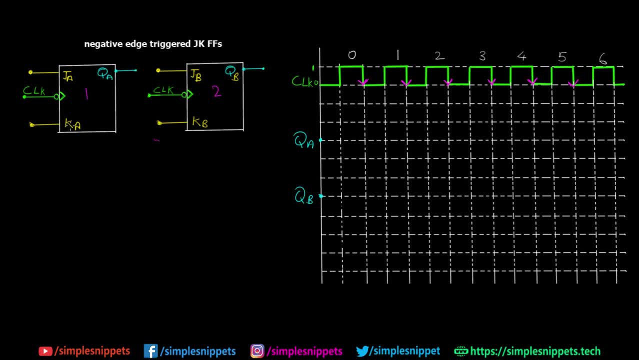 J and K And remember that in JK flip flop when the input is one and one, we get a toggle state right. However, in this circuit you can see there are two different JK flip flops and there is no connection between them. 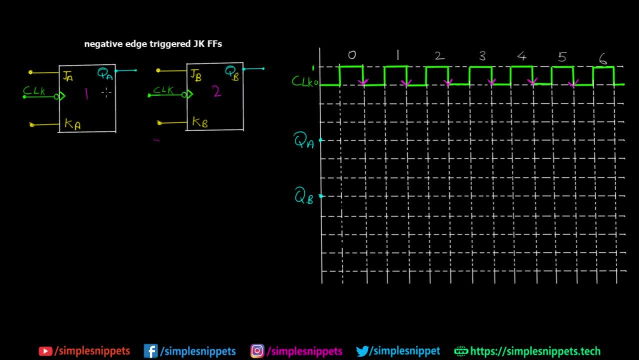 So in order to convert them into a counter circuit, we have to have a certain connection assembly which has to connect these two flip flops, right? So let me just connect them in a particular fashion, and then I'll explain to you what's happening. Okay, So, as you can, 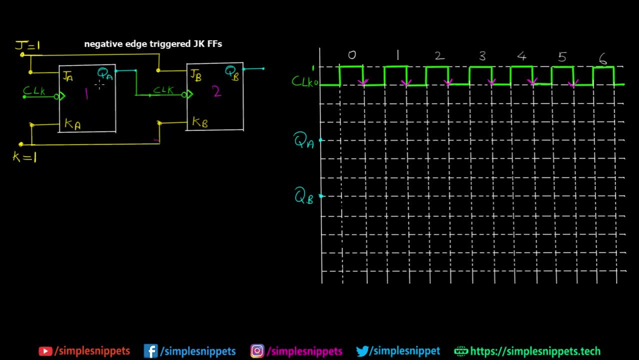 see on the screen. I have made the particular connections. The first thing you'll notice is that output Q a is being fed as an input, as a clock, to the second flip flop. Okay, So we have individual clocks, which means that this is connected in a asynchronous fashion. 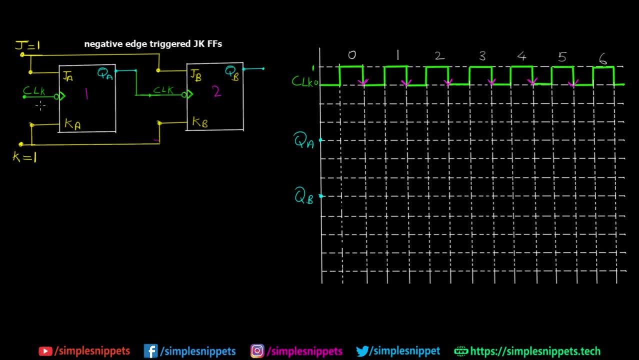 So we've discussed that in asynchronous counters the clocks are different, right? So this is a clock which is individually coming into the first flip flop And the second flip flops clock is actually the output of the first one And the second thing that you can notice 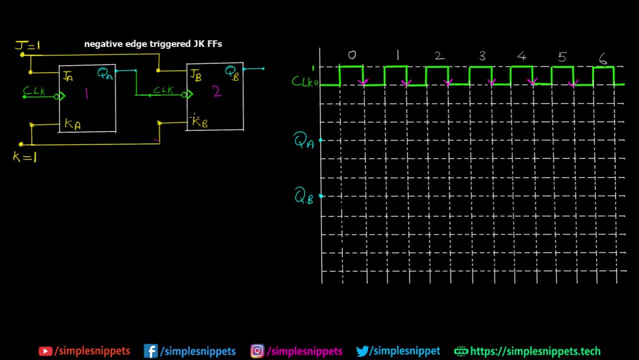 is that J and K is one which is common for both the flip flops, right? So you can see the yellow lines which are connected to both the flip flops, and they are set to one. Okay, So now this makes this entire setup a two bit asynchronous counter, and we'll see how. 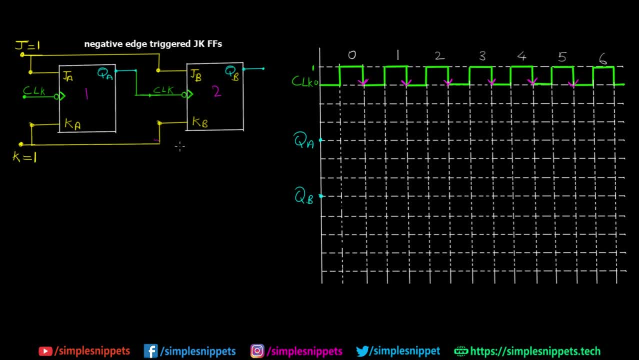 it works also. So now let's try to understand the output of the first flip flop. Okay, So now this makes this entire setup a two bit asynchronous counter and we'll see how it works also. So let's try to understand the output on the clock cycles. Okay, So we are going to be. 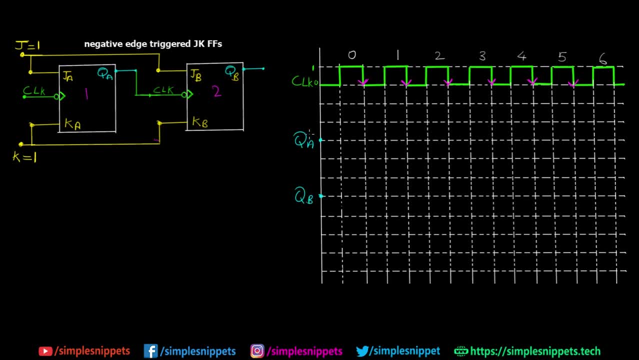 tracking Q a and Q B as the output. So let's see how the values fluctuate. Okay, So I'm going to be assuming Q a initially to be zero, right? So I'm going to start off from zero. So this is zero and this is one. and over here also, this is zero and this is one. 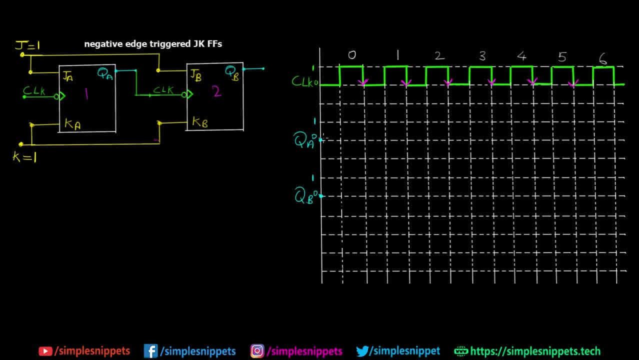 So till the first negative edge comes, we know that Q is going to be zero, only right. So there is no toggling that is going to happen. So till the first negative edge appear. So this clock, CLK, is this one right? 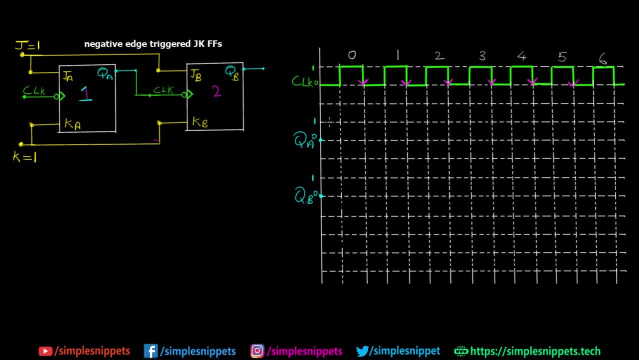 So till the first negative edge, Q is going to be zero, right. So till here it's going to be zero. But as soon as this negative edge happens, the Q a value is going to be fluctuating or going to be toggling from zero to one right. So that's what the toggle state is. 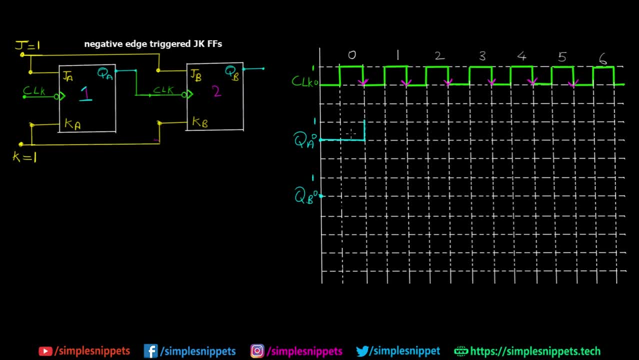 We've seen that in JK flip-flops and in previous videos. and the Q a is going to stay one till the next negative edge, right, So till the clock goes from one to zero, until next time. this is going to stay high in this duration. 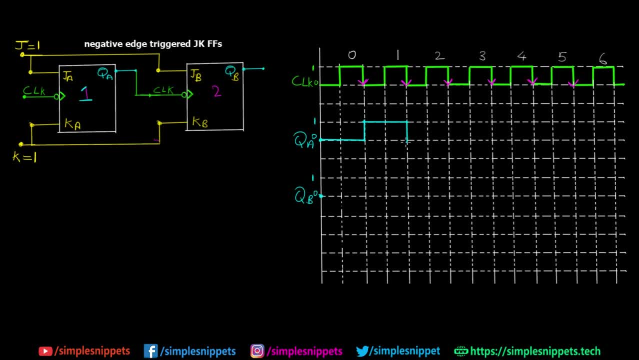 And then, once that happens, it will again drop down to zero. So this is how the toggling is going to happen, right? So let me just mark all the values of Q, a and the toggling that is happening. So every time there is a negative edge, that is toggling happening. 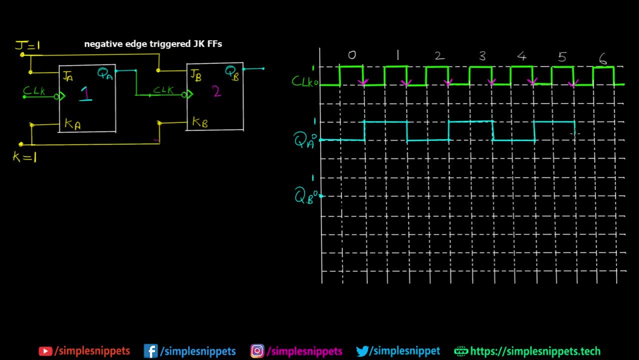 and otherwise it's going to stay stable. So that's how the toggle state works. Okay, So, as you can see, I have marked Q a on the entire clock cycle graph And one thing that you can observe over here is the time period of clock. is this much right? So let's say this: 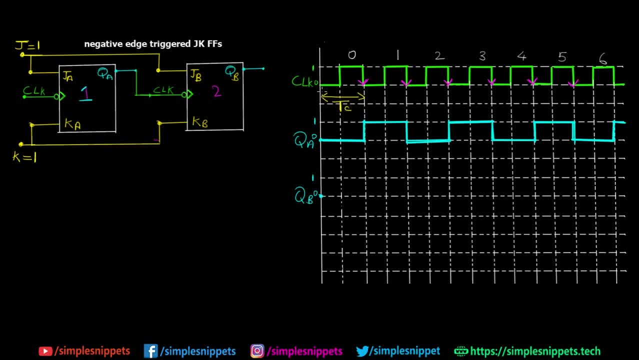 is TC. Let's consider this TC, and I hope you know what is time period. Time period is one complete full cycle. So I've marked the first one as zero. Then this is the second complete full cycle of the clock. Again, this is also TC. So the time taken by the waveform to complete 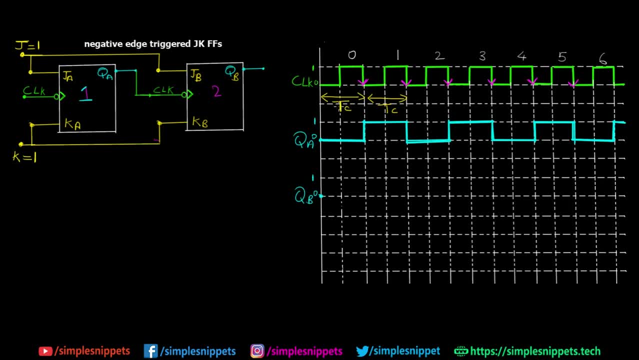 one complete cycle is known as the time period of that waveform. So you can see this is that time taken by the clock. Okay, Now, if you observe, the time period for Q, a is twice right. So let's say this is TA. 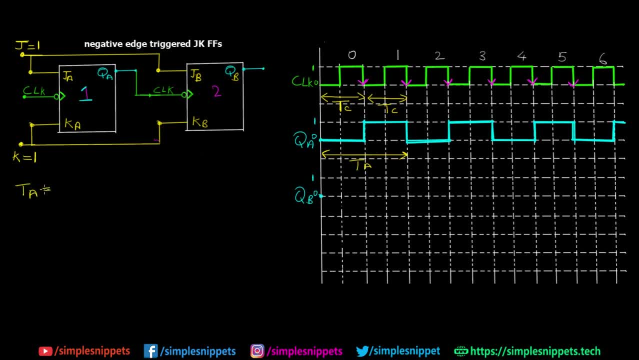 So by looking at the graph you can see that TA is equal to two times of TC, right? So this is clearly visible in this chart also. So if we see the frequency, if I say FA, then it will be exactly opposite, right? So it will be FC by two, because time period is inverse. 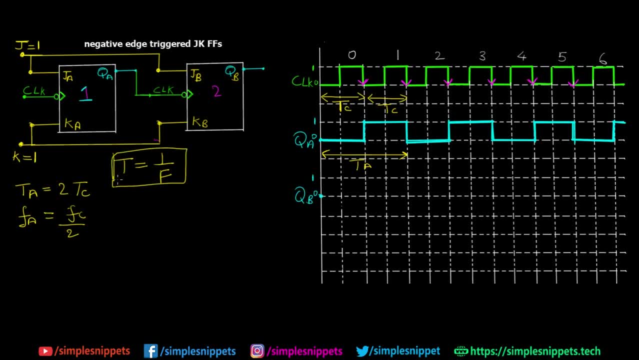 to frequency, right? So you've? you've probably studied this formula many times in your physics, in your mathematics. So time period is inverse of frequency. So this is something which is very common and basic. So here you can see that FA is one by two of FC. or you can also say FC is two times. 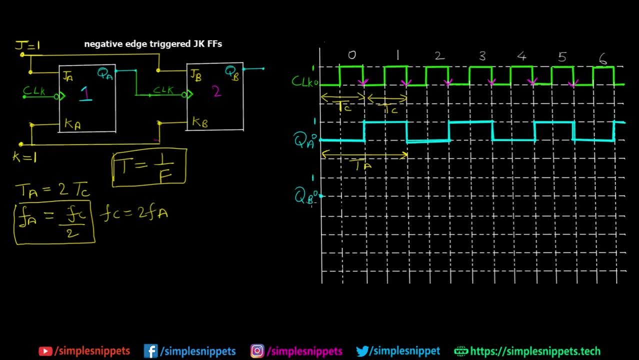 of FA. right now, Let's try to track QB now. Okay, So this is the second output of the second flip flop. up until now, we've tracked only QA. Okay. So again, even this flip flop is negative edge trigger flip flop. However, if you see the clock provided to the second, 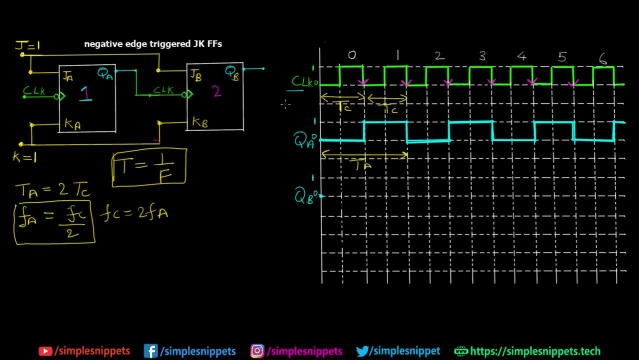 flip flop is basically the output of first flip flop, QA. So we're not going to be considering this clock, but we're going to be considering QA and QB As the clock for QB right And for QB, since being negatively edge triggered, it will get. 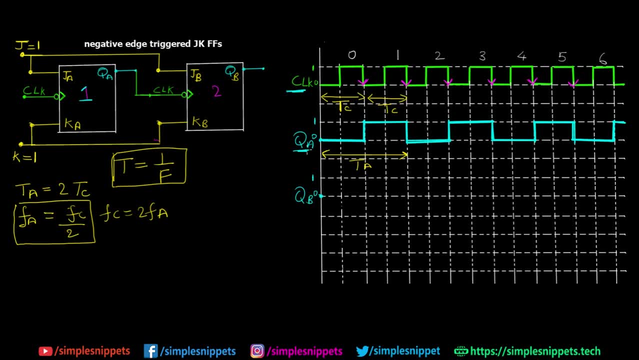 activated on negative edges of QA. only right, So let's mark the negative edges of QA over here. So this is the first negative edge, This is the second negative edge, This is the third, and then we'll have them more when we move ahead in time. But right now, let's 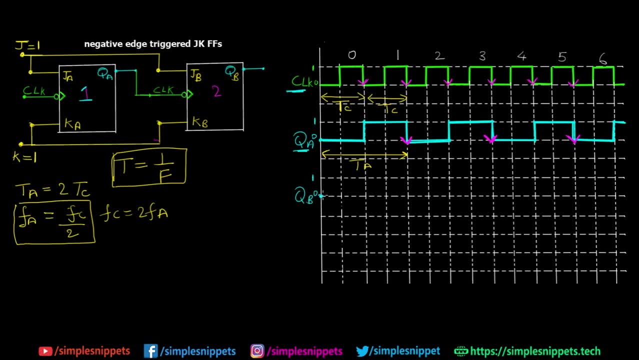 calculate only these three negative edges. So again we are starting QB from zero. Okay, So of course QB is going to stay zero until the first negative edge. So over here we're going to have the first negative edge of QA. So this is the first negative edge of QA. 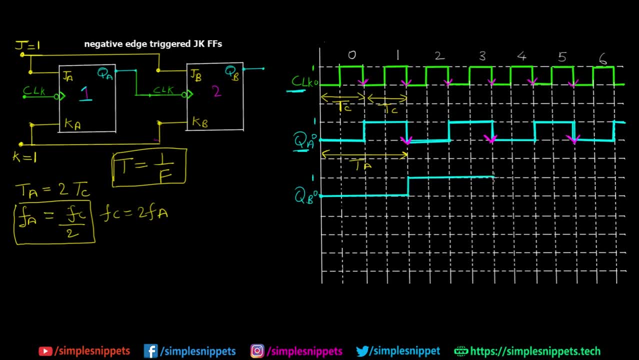 So that's when toggling is going to happen, And then it's going to stay one till the next negative edge, So till the second negative edge of QA. So again it will get toggled back to zero. Then again it will stay low till the third negative edge till here, and 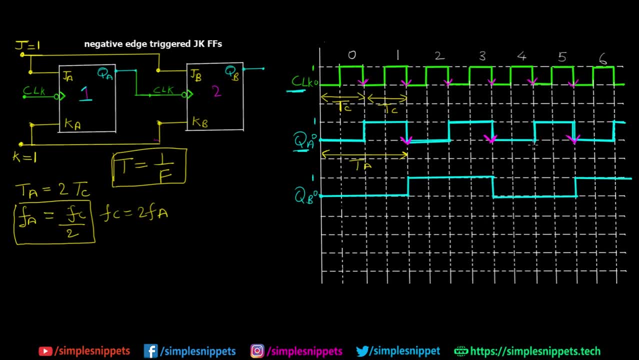 then it'll again get toggled back, Okay. So now again we are having a new observation over here, and now you can see that the time period has again doubled right. So if you see, this is the new time period of QB, So you can consider this as two negative edges. 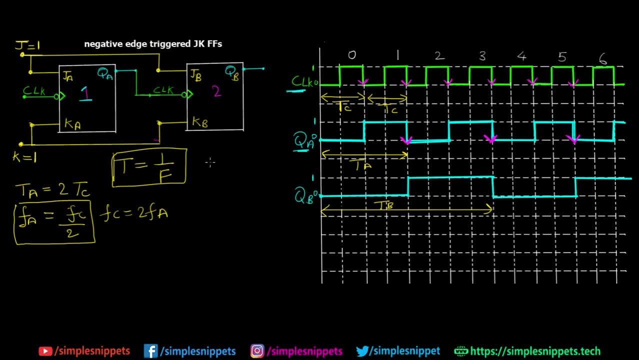 T of B and you can clearly say that T of B is twice of T of A, right? You can see it from the graph, which essentially means that T of B is four times of T of C, right? So four times of this- So one, two, three and four- is equal to one time of T of B, right? 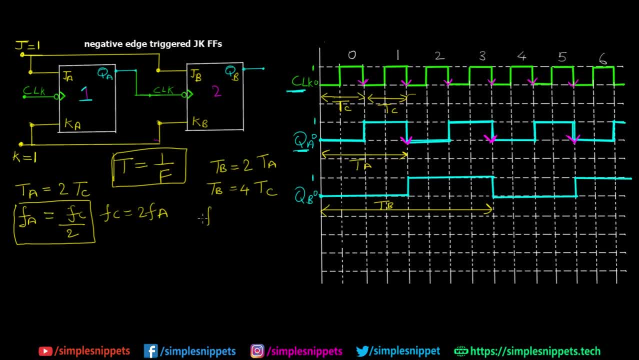 You can again observe this from the graph itself. So this means frequency of B is equal to frequency of clock by four. or you can also say F of C is equal to four times of frequency of clock by four. So this is the frequency of clock by four. So this is the. 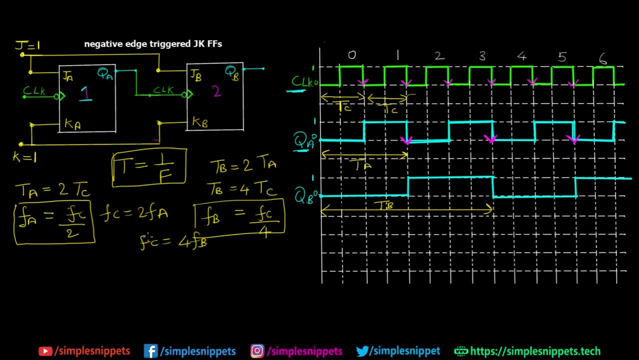 frequency of B, right? So you can make these deductions. Now, here you can notice that there is a pattern in the frequency and time period, right? So every time a new flip flop is going to be added, the time period is going to get doubled and the frequency is going to get. 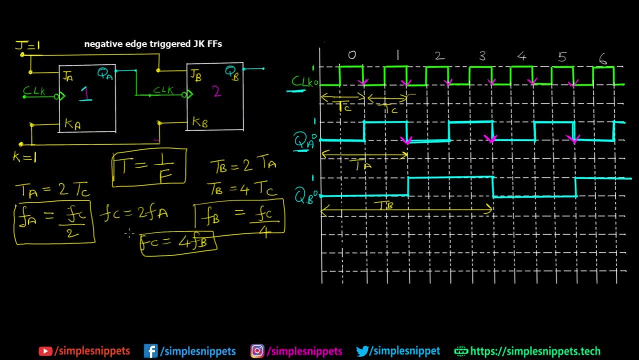 divided by two right. So there is a generic formula. So if there are N number of flip flops, the time period is going to be two raised to N and frequency is going to be one upon two raised to N of the original clock right. 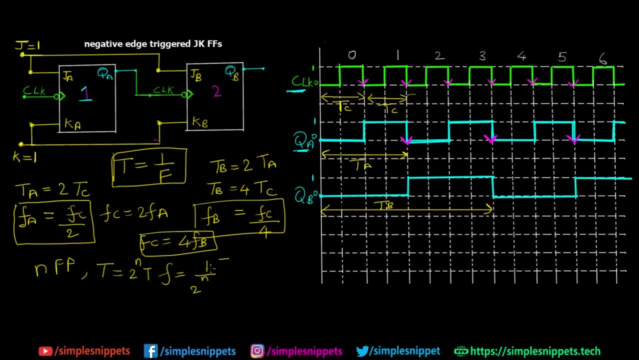 So let me just erase this out. So yeah, this is the formula that I was seeing. and let's say, you have four flip flops, right? So if you have four flip flops in this particular fashion, where J and K is common and the clock of the next flip flop is the output of the, 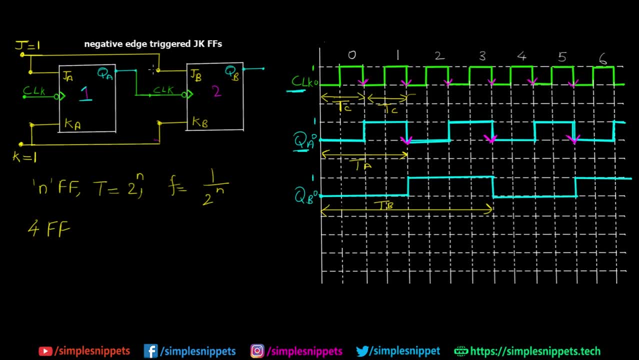 previous flip flop. So in that case, this entire circuit is going to act as a asynchronous counter as well as a frequency divider Which divides the frequency every time by two and multiplies the time period every time by two. Okay, So if we have four flip flops, the frequency F of four, the frequency of 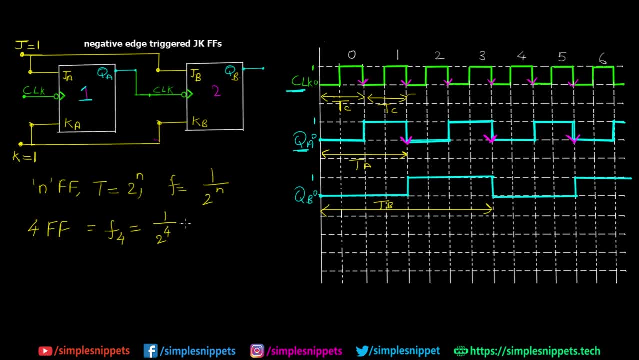 the last flip flop is going to be one upon two, raised to four, which is going to be one upon 16 times that of the first flip flop, Okay, Of F of one, And the time period is again going to be 16 times more right, Because at every stage it is getting doubled. That 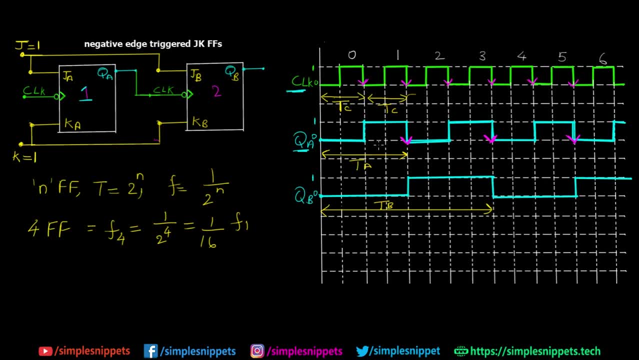 is the time period is getting doubled and frequency is getting halved, right, Okay? So this is one deduction and this is not basically counting. This was something else that I wanted to talk about, but now let's see how this counter circuit is going to perform. the actual 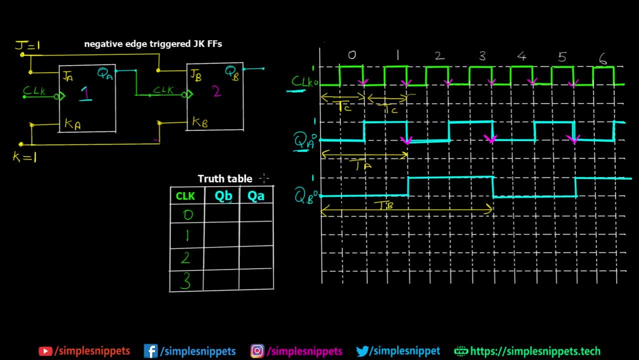 counting, Okay, Okay. So, as you can see on the screen, I have a new table over here And what I have over here is the clock signal, this the first clock, and then the signal counts. So this is the first cycle. This is the second cycle, So I've started from zero. 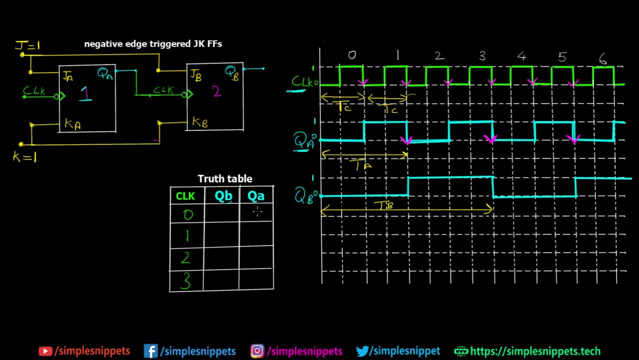 one, two and three, because you're starting the counting from zero over here. That's why I've started the counting. I've started the counting of the cycles as zero, one, two, three, four and so on. Right, So that's what I have over here, And then what you're measuring is the values of QB. 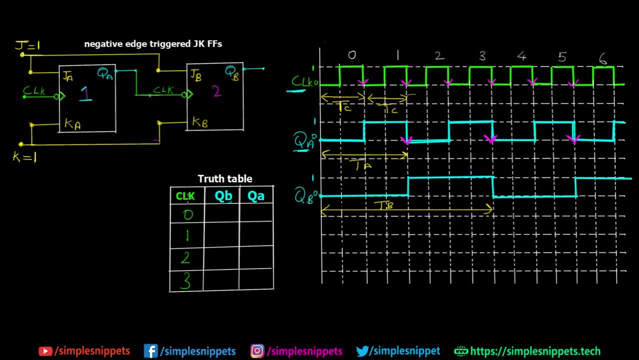 and QA. Okay, So let's see what happens at clock of zero. So in four cycle, this entire time duration, you can see QA or zero and you can also see QB was zero, right? So let's just put those values over here. Now let's see what happens at clock cycle one. So at 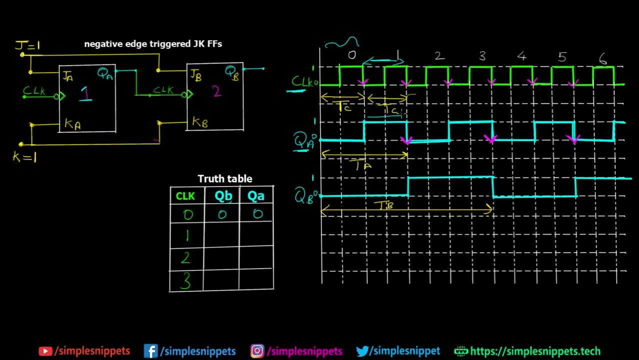 clock cycle one, which is this part: Sign. here you can see that QA was one. However, QB was zero. right, In this part, QB is still zero. Okay, In clock cycle two, which is this part you can see, QA has become zero. but. 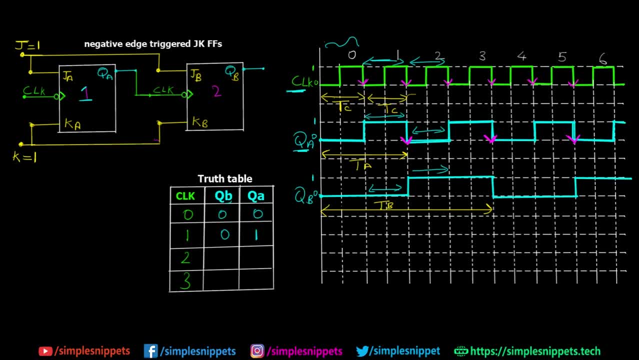 now QB is one. Okay, Mr Double warrior, yeah, QB is one and QA has become zero. And now, if you observe the last case where in clock cycle three- which means that we are in this period- QA is when, then QB is also one. so one one, And now I'm going over here. So 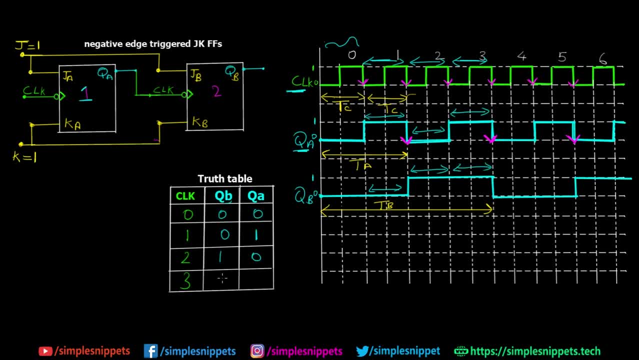 where it the number one, number one. now notice these digital values. so 0: 0 stands for decimal of 0, 0, 1 stands for decimal of 1, 1, 0 stands for 2 and 1: 1 stands for 3. so this exactly is what i mean by counting. and if you 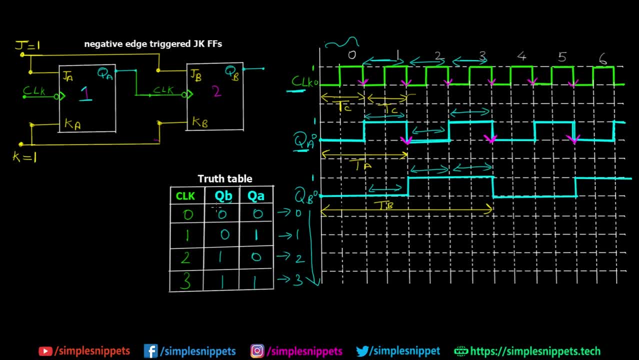 again move ahead from the third cycle to the fourth, you'll again get these repetitive values of 0, 0, 0, 1, 1, 0 and 1, 1. you can go ahead and count ahead, but the reason why you'll get repetitive values is because our 2-bit counter over here can only count 4 values, starting from 0 to 3, and 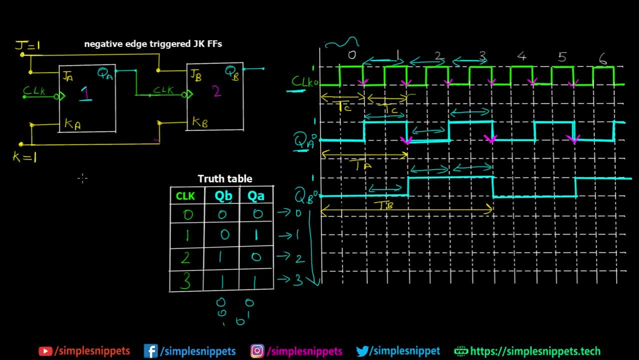 the reason why it can count only 4 values is because we are using 2 flip-flops. so again, there is a formula which is 2 raised to n times the numbers it can count. so this n represents the number of flip-flops. so since we have 2, 2 raised to 2 is equal to 4, so we can count from 0 to 3. 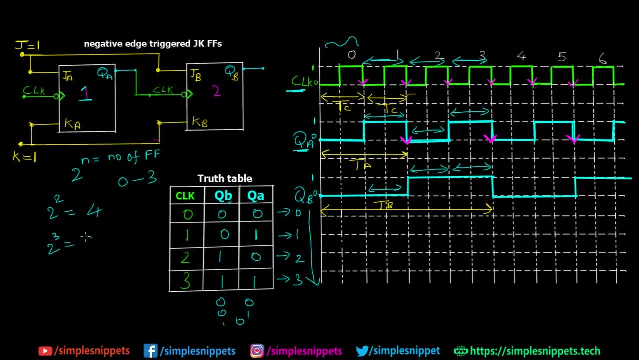 so if we add one more flip-flop, it would be 2 raised to 3, which is equal to 8, so we'll be able to count 8 different values, starting from 0 to 7, right? so there would be qc over here and then all these values would be. 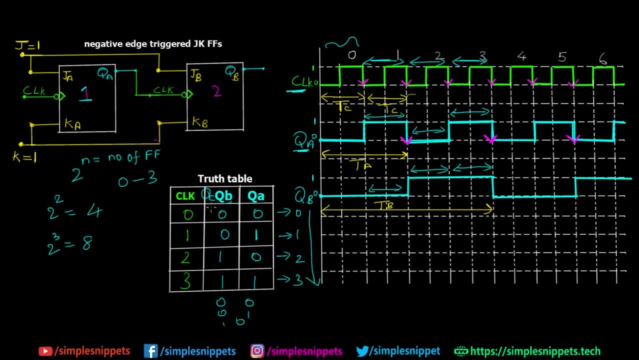 something like 0, 0, 0, 0, 0, 1 till 7. okay. so yeah, this was how the counters count the actual digital pulses, and i hope this is very clear now from the entire clock cycle diagram and from the assembly. so this was a very basic counter with a synchronous connection and it was just a 2-bit counter which 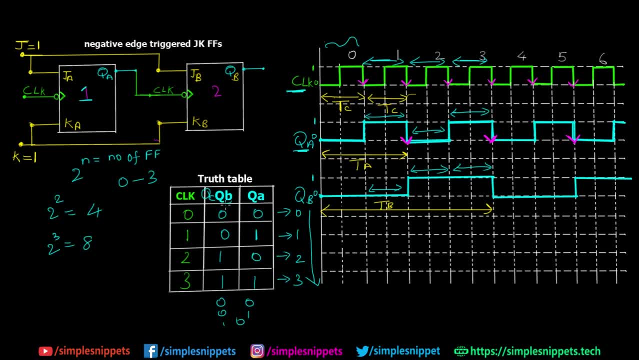 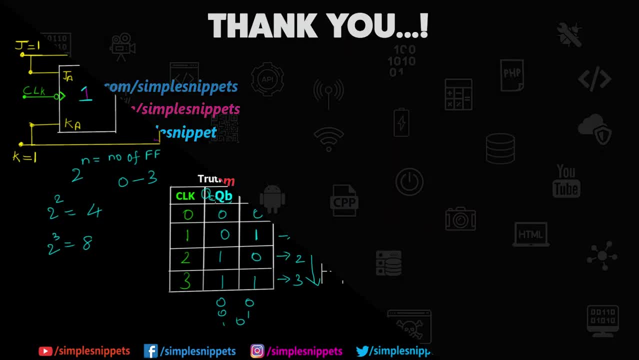 was counting four different values, and i hope it is clear now, and in further videos we'll see how to count the actual digital pulses. so this was a very basic counter with a synchronous connection, and then we'll see different types of counters: synchronous, asynchronous and then depending upon their sizes also. so, yeah, that's it for this video, guys. i hope you understood the. 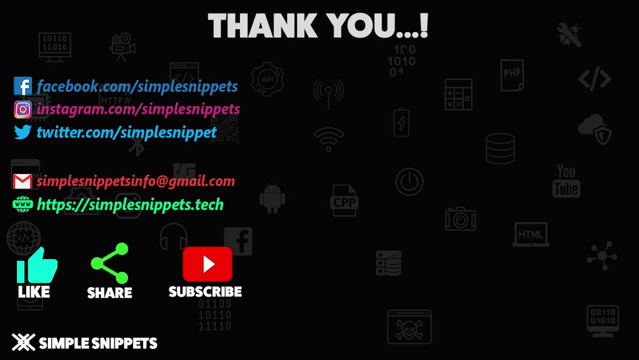 concept of counters now, practically and visually, how they actually count the values and pulses. if you like this video, please give it a thumbs up, share it with your friends and, if you haven't subscribed, make sure you subscribe to this channel because you'll get notified whenever i upload a new video tutorial, just like this or some other information technology. 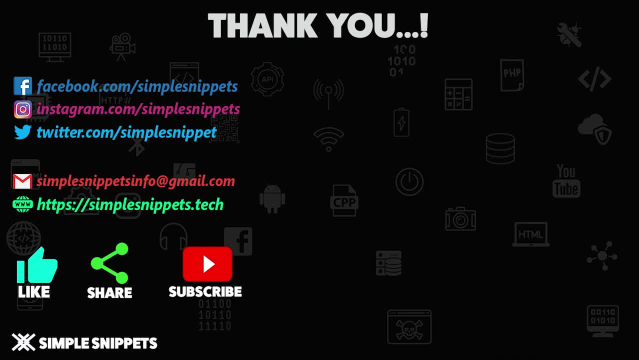 oriented topic. thanks for watching, guys. i'll see you guys in the next video tutorial. peace.